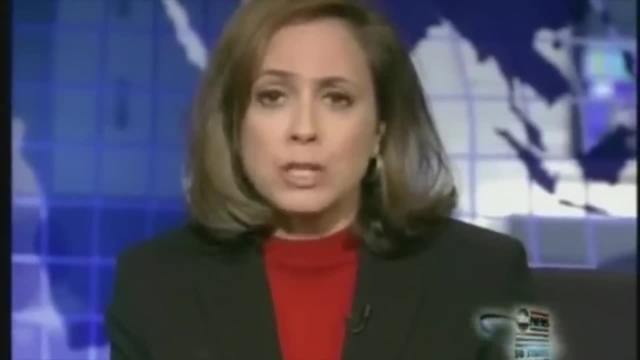 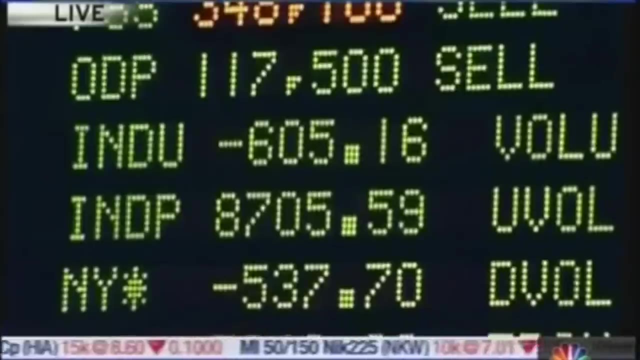 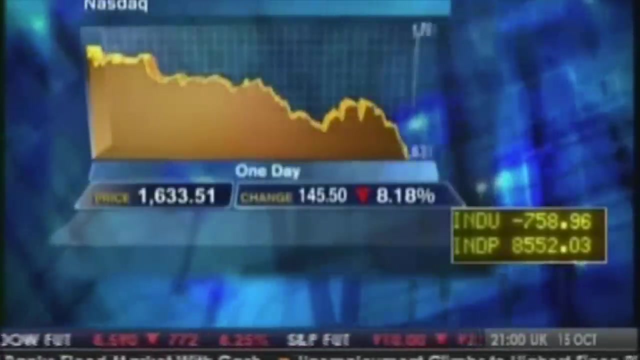 18%. The stock market is now down 21%. Because we're now down 14%, 33%. What in the world is happening on Wall Street? Two-year no yields went from 190 to 166 in the blink of an eye. The NASDAQ, everything and more, has been completely wiped out It. 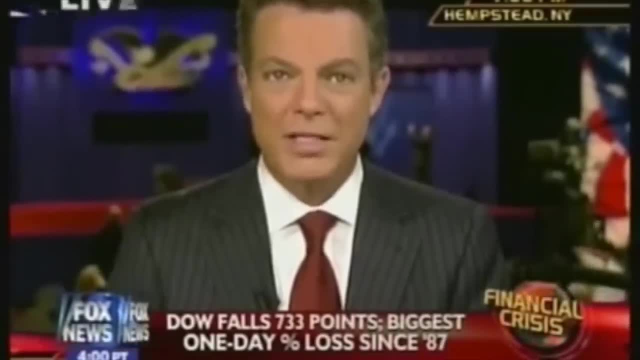 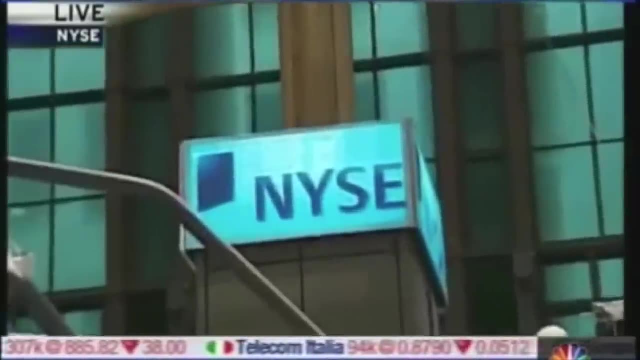 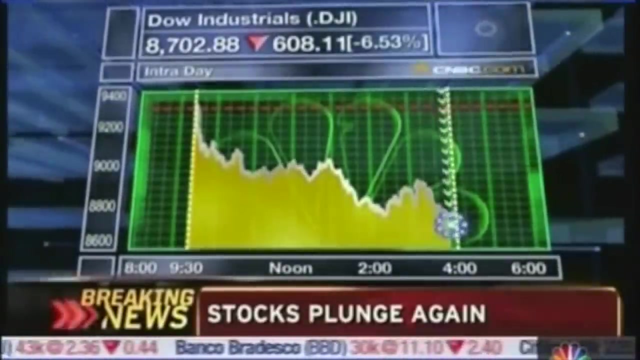 was the worst day on Wall Street since the crash of 1987. From the financial capital of the world, the opening bell is going to ring in five seconds And, to be honest with you, we wish it wouldn't. Traders here working the phone say a lot of their customers are. 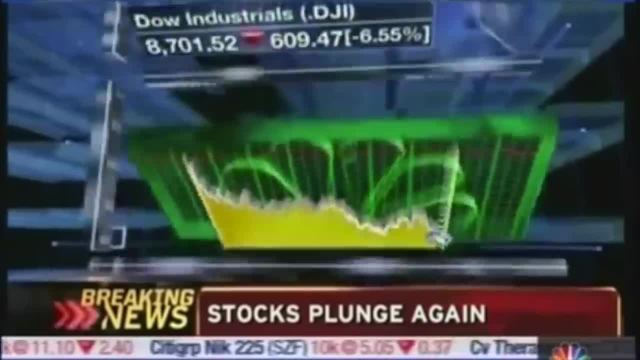 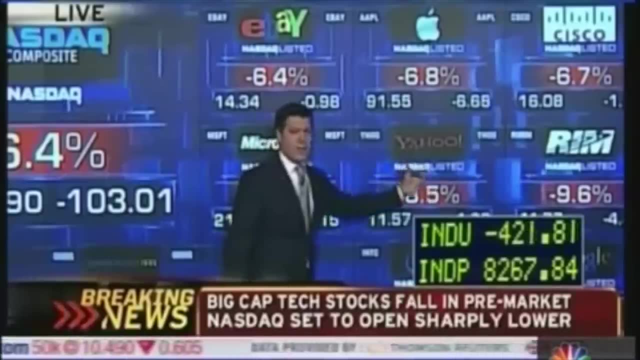 freaked out. We're waiting to see how low the Dow will go. They're focused on the Dow, not so focused on OPEC. Yes, OPEC did cut production by one and a half million barrels per day. Really, you're seeing just broad-based declines across all of the major technology sectors. 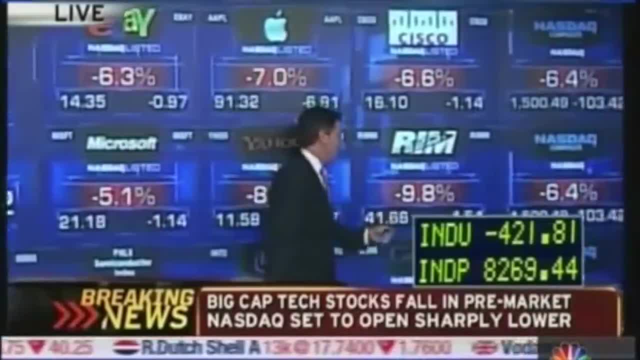 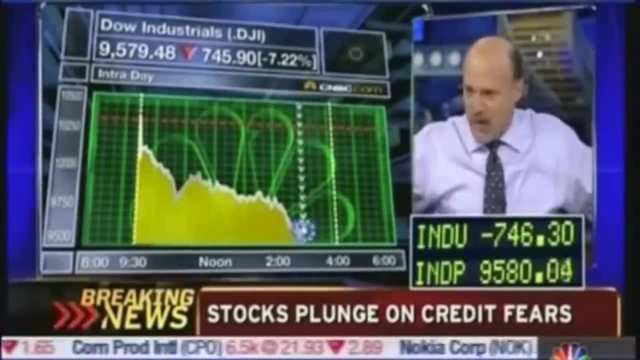 Apple's under pressure. Yahoo down 8.5%, Cisco 6.5%, Research in Motion 10% And we're not getting the bid wanted. We're not getting the stop trading and we see where the buyers are. We're just every day they're pounding it. 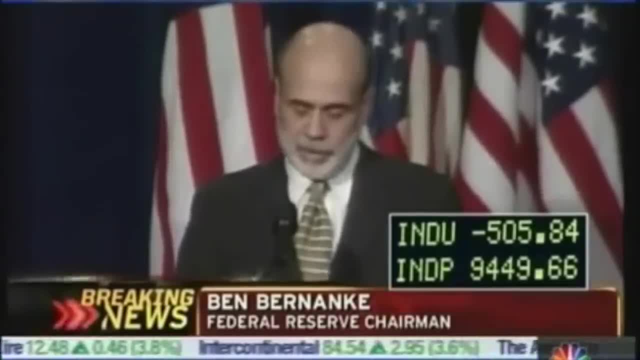 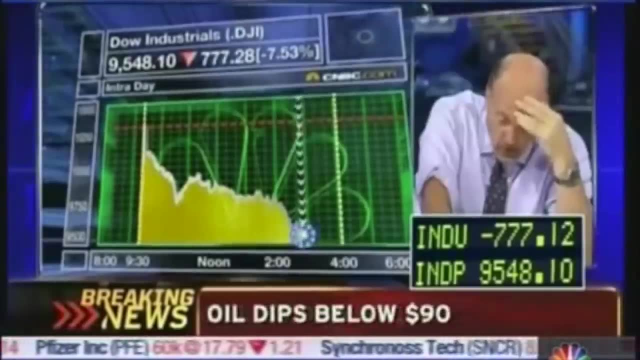 The heightened financial turmoil that we have experienced of late may well lengthen the period of weak economic performance and further increase the risk to growth. Can't look at it after you buy it. It's so horrible. We've had an eight day losing streak in the Dow. that, in percentage terms, puts it on par. 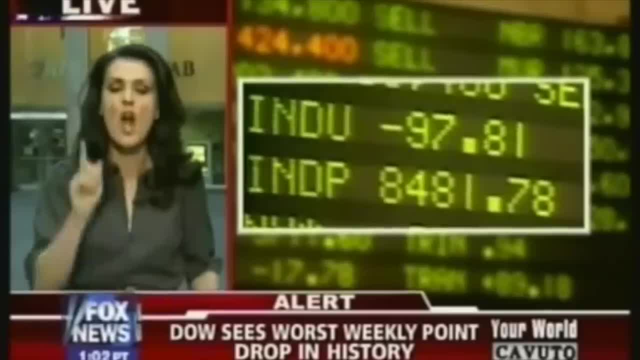 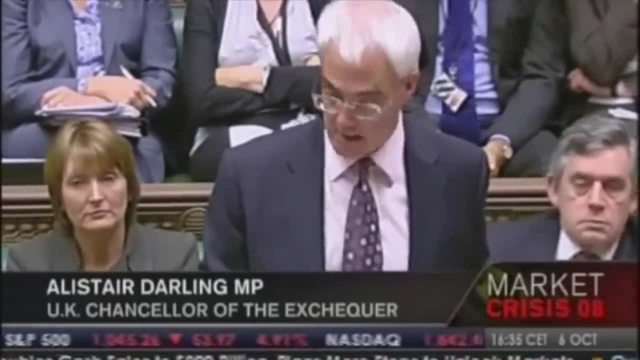 close to the loss suffered in that crash in 1987, close to that percentage loss those two days in 1929.. What started in America last year has now spread to every part of the world. We're down 9% today. The Zetra DAX over in Frankfurt is down by 9%. The Paris market: 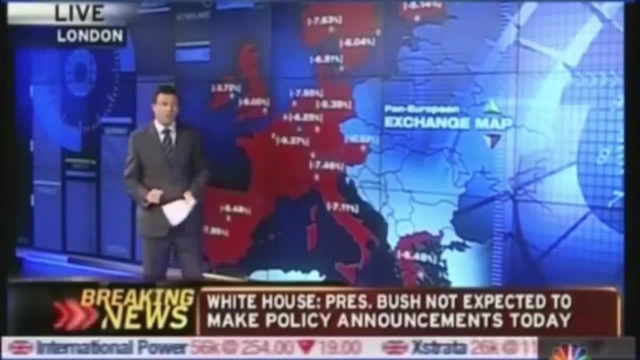 down by 9%, Austria is down by 9%, The US is down by 9%, The US is down by 9%, The US is down by 9% And Austria, which was briefly suspended earlier on in the day, is. 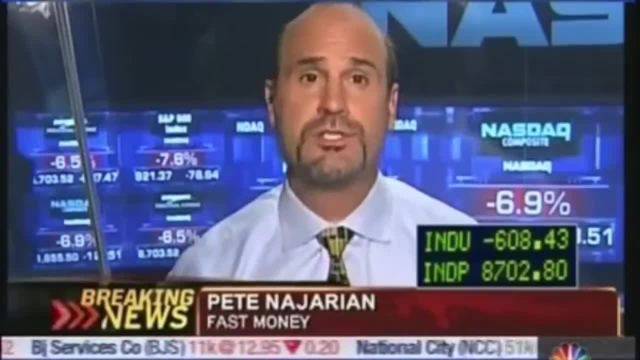 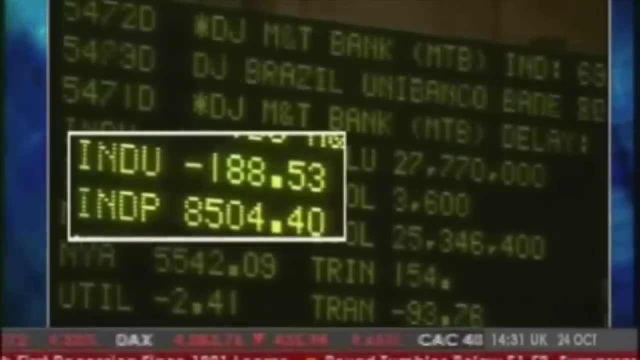 down by nearly 11%. This market is as volatile as you'll ever see. Traders saying this is the craziest day they have ever seen in these markets. Veteran traders saying they've never seen anything like it. The movement in oil prices so fast. so 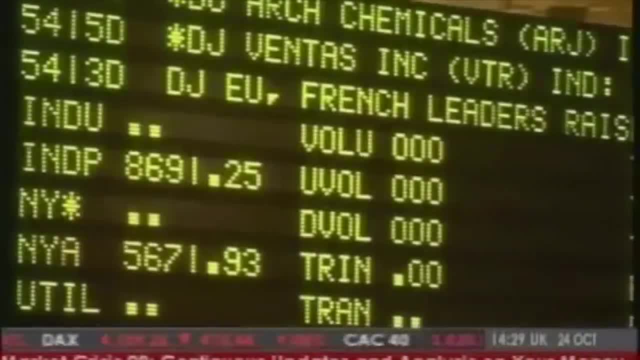 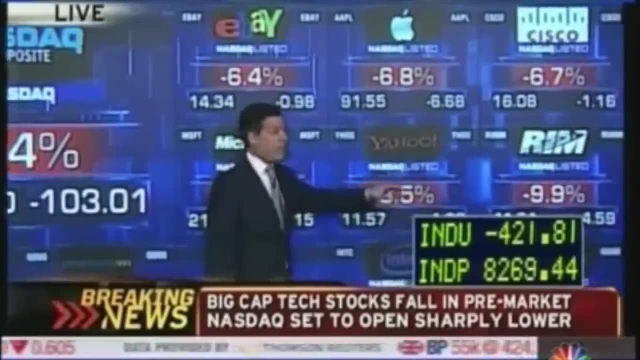 Seconds ago until the start of trading at the New York Stock Exchange and stocks are set to kick off lower, a whole lot lower. eBay is down 6.5% and really you're seeing just broad based declines across all of the major technology sectors. 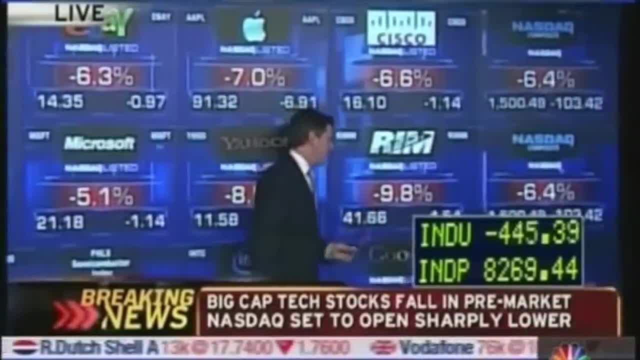 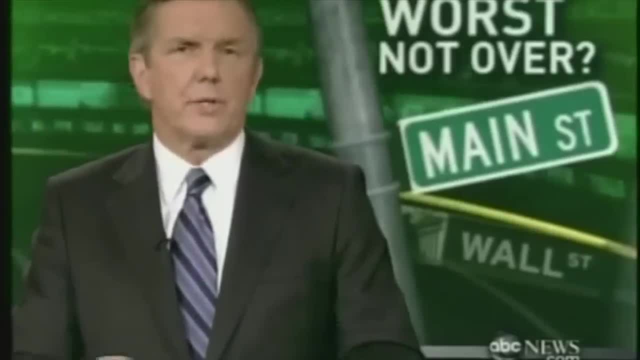 Yahoo down 8.5%, Cisco 6.5%, Research in Motion 10%. This could be the most serious recession in decades, And that means life as most Americans know it is about to change, in some cases dramatically. 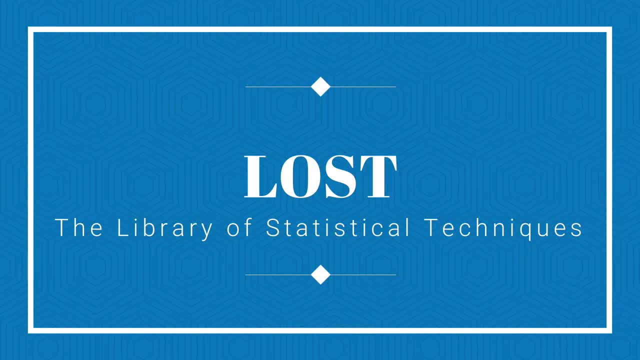 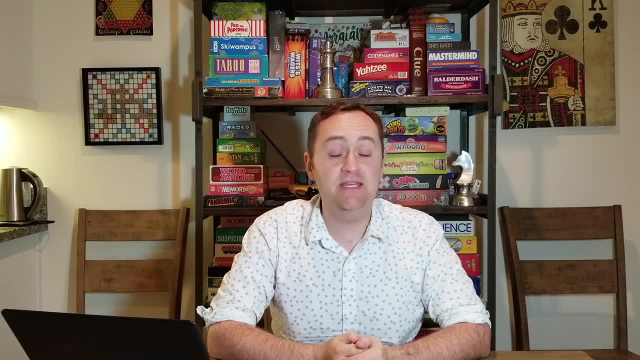 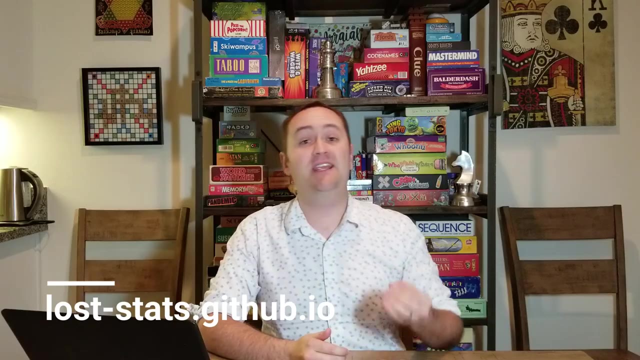 Hello, my name is Nick Huntington-Klein and I'm here today to talk about the Library of Statistical Techniques, or LOST. LOST is a publicly editable website designed to make it easier to figure out how to perform particular statistical techniques, such as doing some sort. 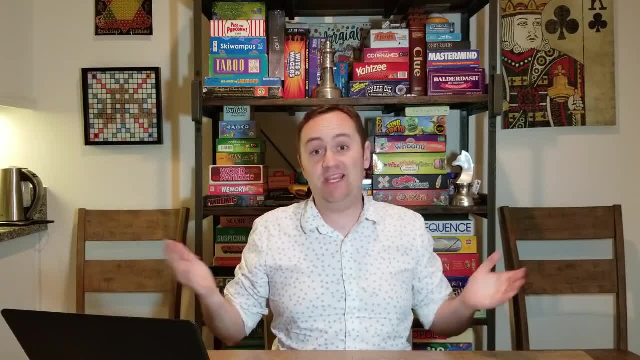 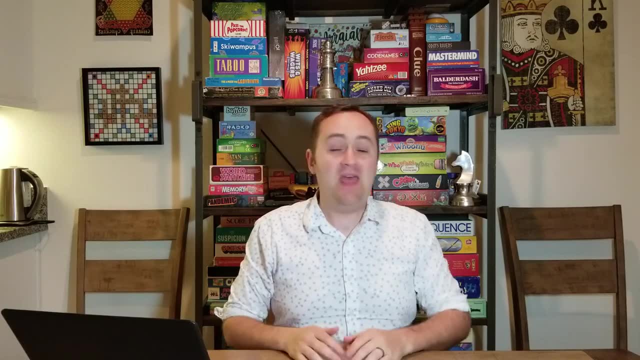 of model estimation or data manipulation or data visualization in your software or programming language of choice. It is a publicly editable website, like I said, sort of like Wikipedia, and that means that it is a great place to learn about how to perform statistical techniques. 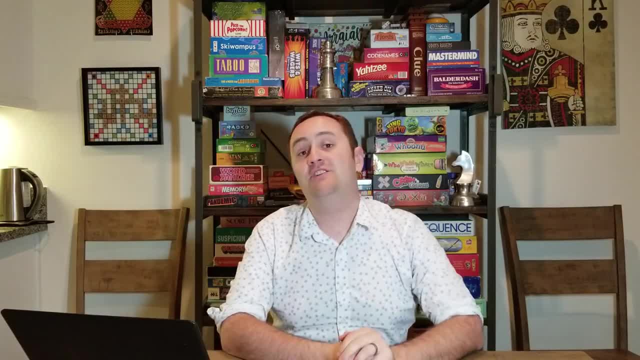 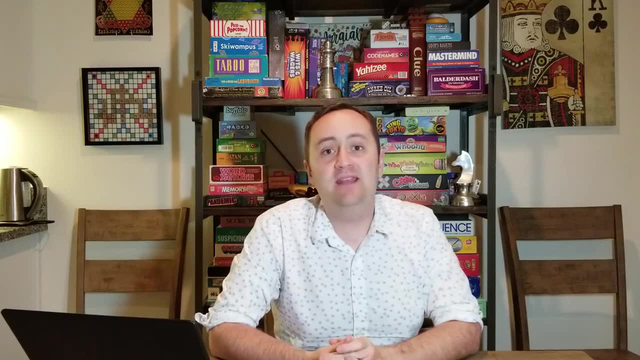 but it's also a great place for you to be able to contribute the knowledge that you have, and this video is going to focus on how to contribute to LOST. Of course, you can also just check it out and see what you can find. You can visit the LOST website at lost-statsgithubio. 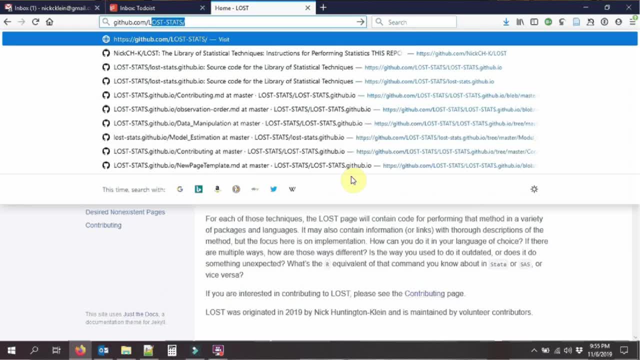 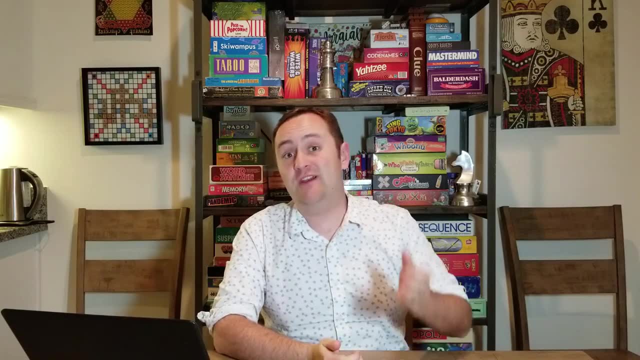 or you can also visit the LOST GitHub repository and then you can figure out what's going on behind the scenes. So let's say that you've looked around the LOST website and you think it might be kind of interesting and you are interested in contributing. Let's talk about how you can do that. 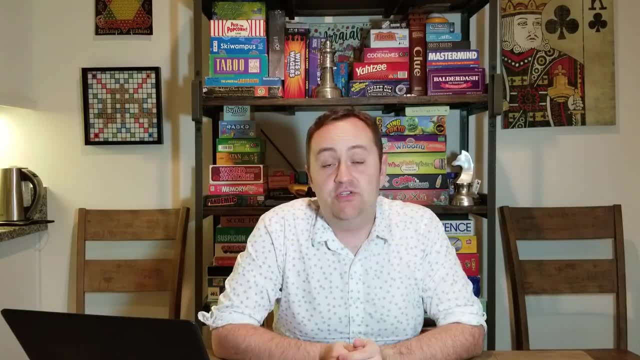 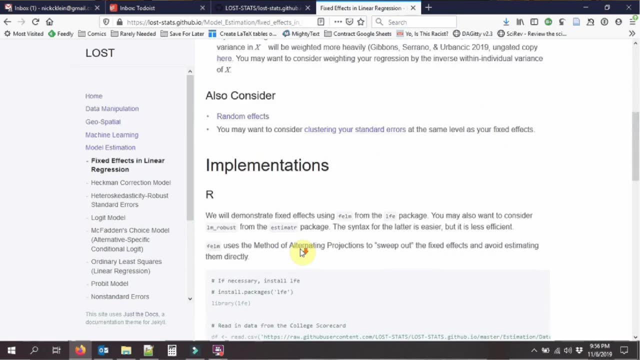 So the first thing that you're going to want to do is figure out what it is that you would like to contribute. I would recommend looking around the pages that already exist. Maybe you find something, an error, that you can correct, or a method that's being used that maybe you can. 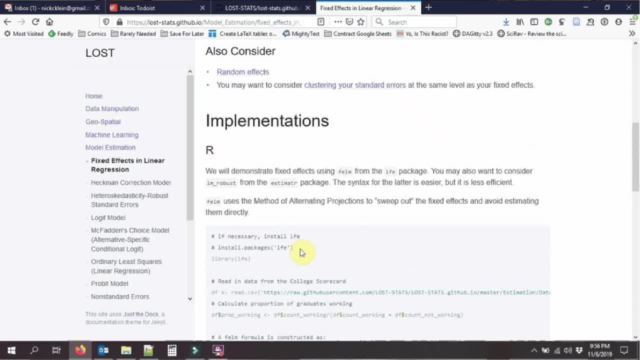 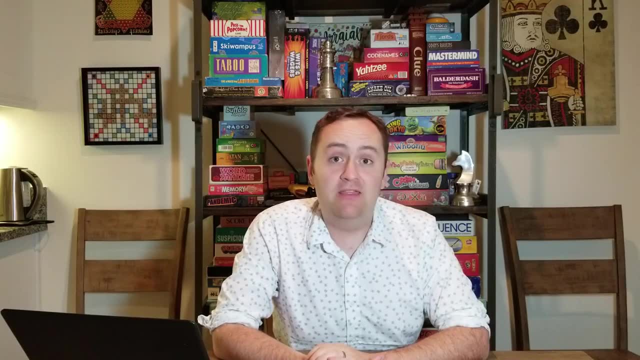 improve upon, or there's a language that is not present on one of the pages that you can fill in. Maybe someone before you has already written how to do something in Stata and you want to write about how to do it in Python, Or you can find a page that needs to. 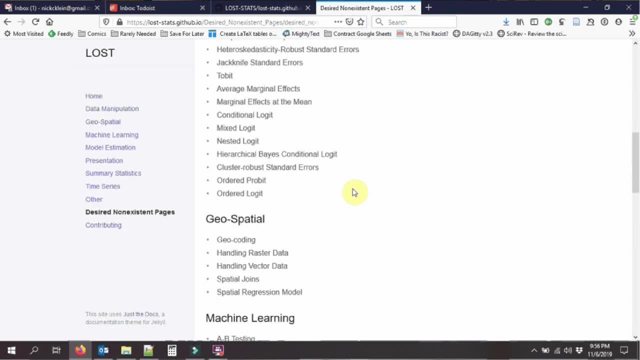 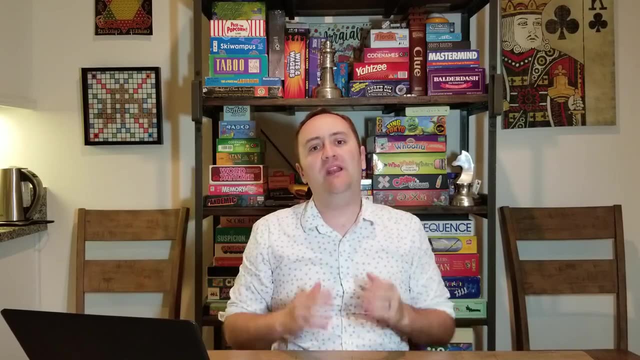 exist and doesn't already. On the LOST website, there is a page called desired non-existent pages, which might give you a couple of ideas of pages that you could create all your own, Once you know what it is that you want to write. well then, it's going to be time to write it.